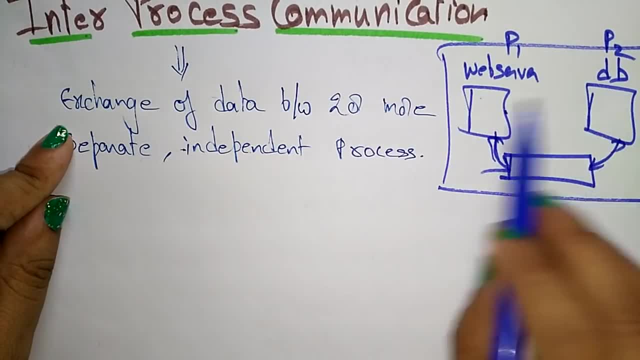 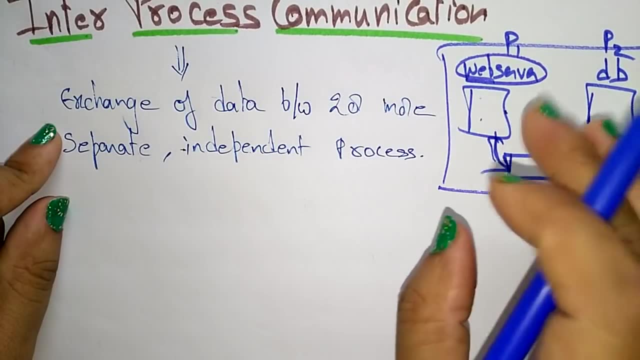 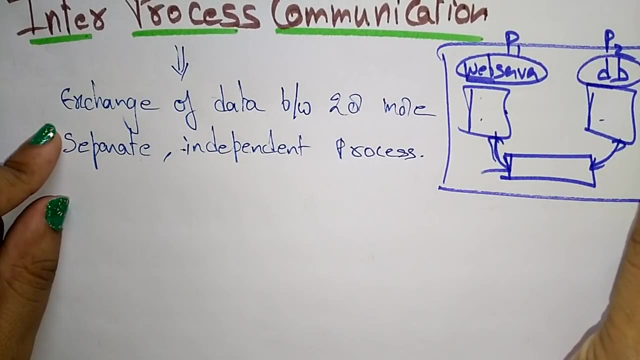 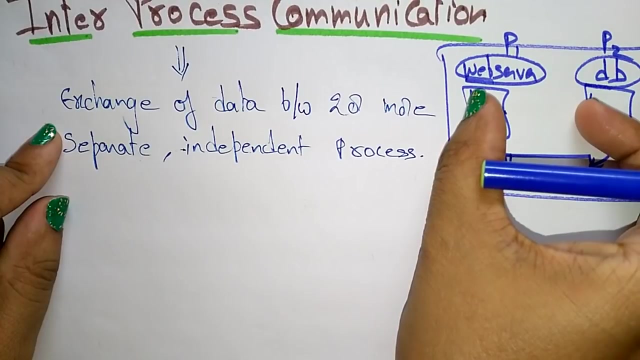 So here we are exchanging of data between these two processes. So these are the two processes which are separate and these are independent. So the web server is having their own ID and it is having their own IP and the same own address, And whereas for the database is also having their own identification. So these two are the independent process, These are the two independent process and these two independent process wants to exchange of data. So that technique you call it as a inter-process communication. 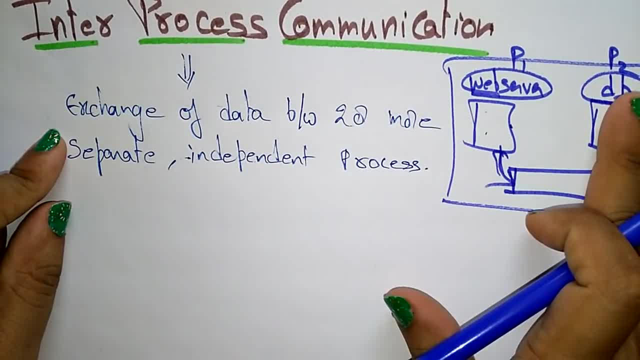 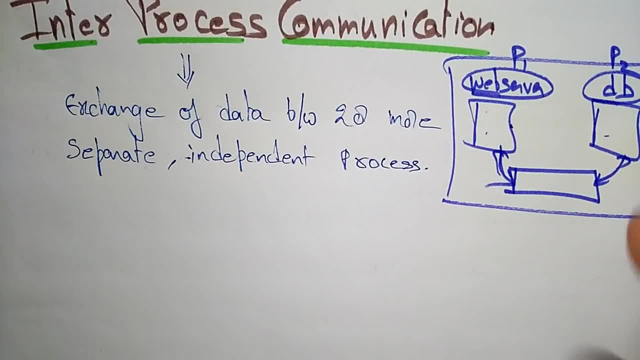 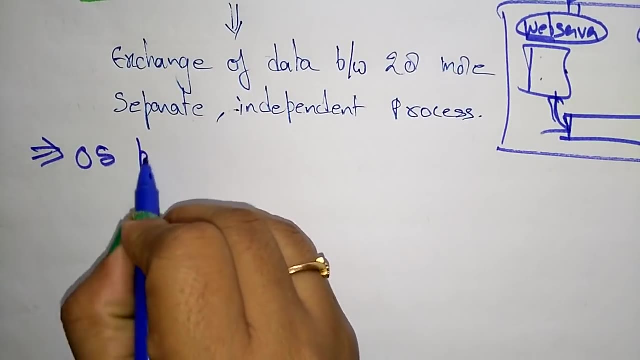 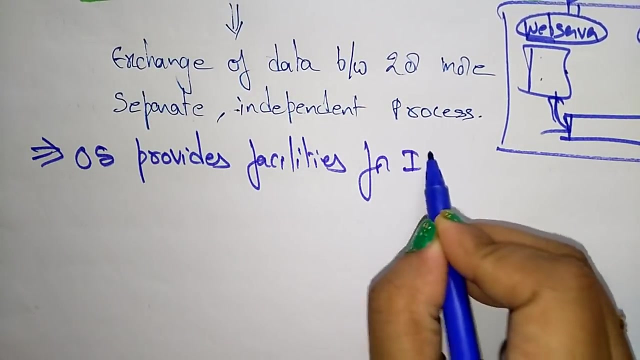 So this one process and another process, So the communication between the within the system. you call it as inter-process communication. So this operating system provides the main, this operating system, whatever the operating system you are taking, that operating system provides facility for inter-process communication. 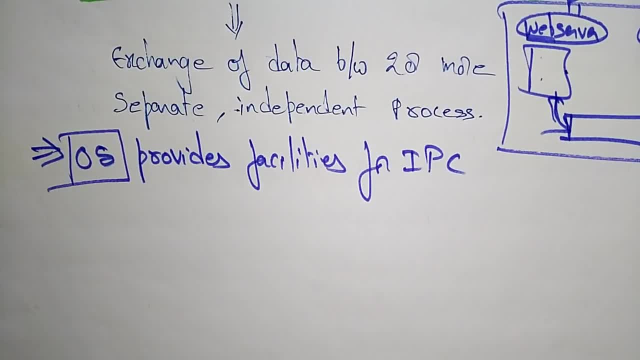 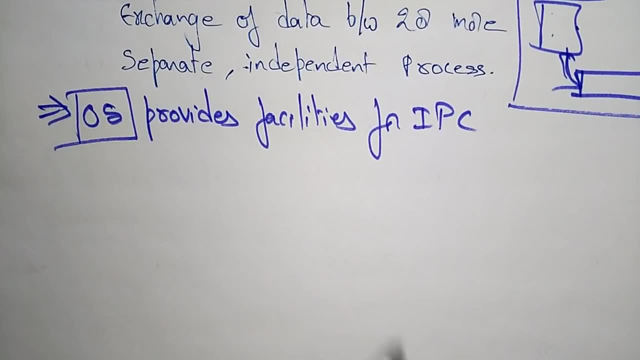 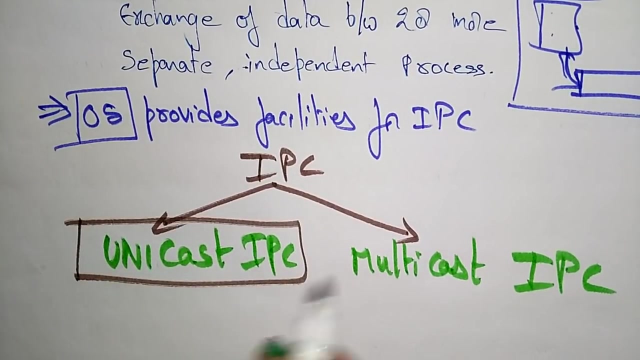 So main this operating systems that provides the facilities for this inter-process communication. This inter-process communication is divided into: inter-process communication may be a unicast. It may be a unicast or it may be a multicast- Multicast, inter-process communication. Okay, the inter-process communication may act as a unicast or it may act as a multicast. 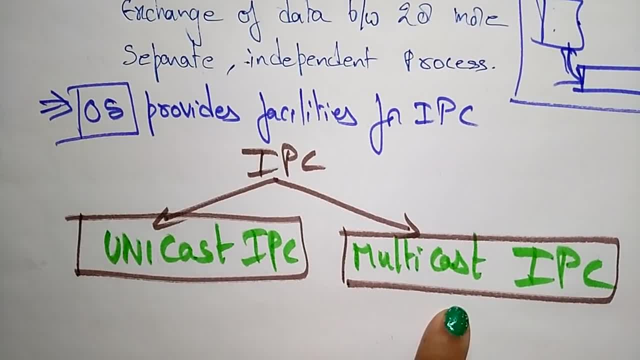 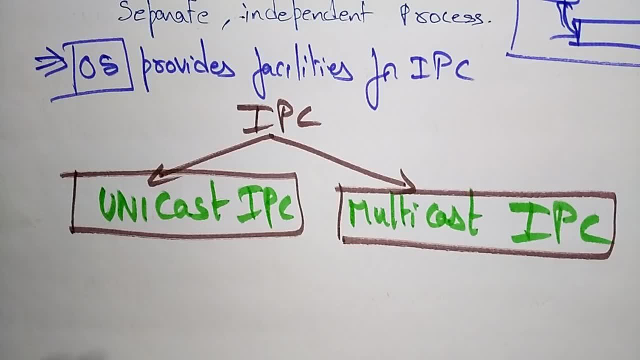 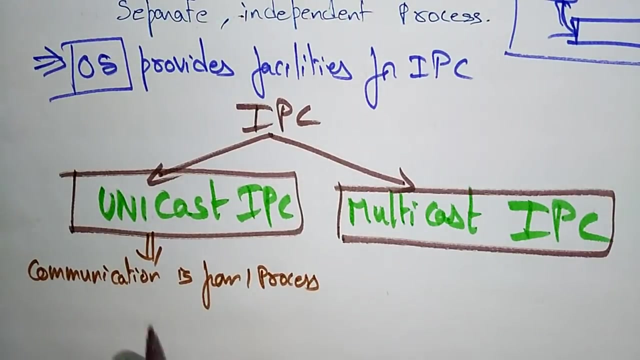 So what is this unicast inter-process And what is a multicast inter-process? Actually, unicast is a communication is from one process to single other process. That you call it as a unicast. What it mean- A communication is from one process- means from one process to single other process. 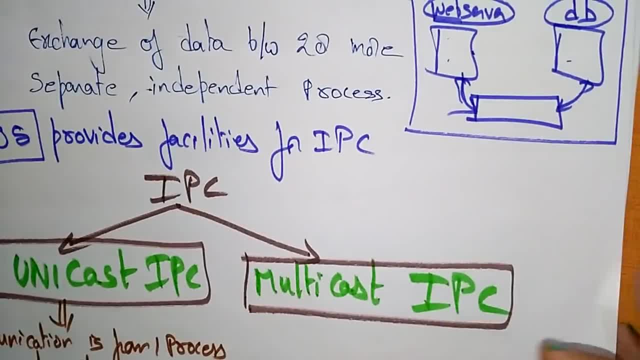 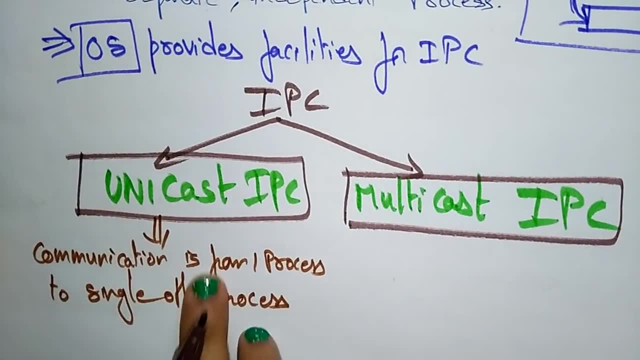 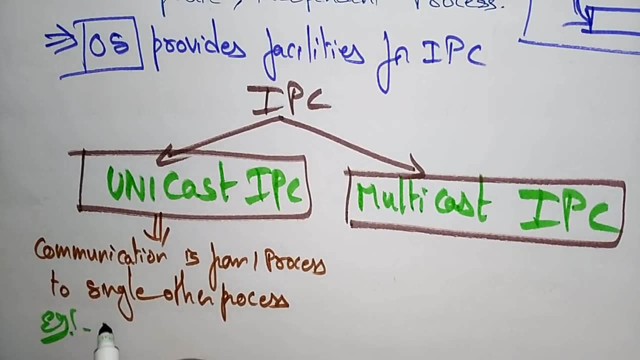 That you call it as uniprocess. So here this case is a uniprocessor. So here one process is to single other process. This type of communication you call it as a unicast, inter process communication. So the example for this unicast, inter process communication is: let us take the socket communication. 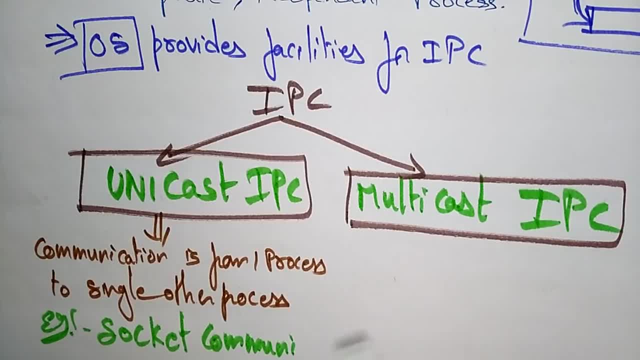 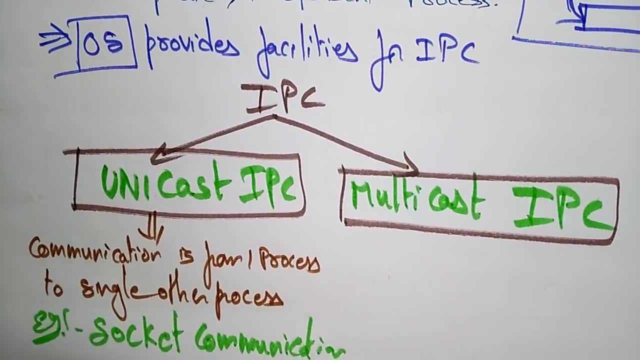 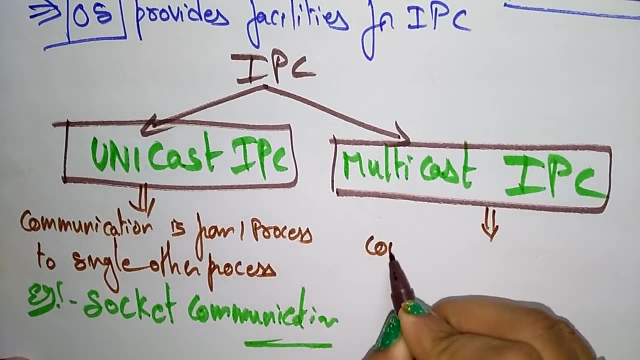 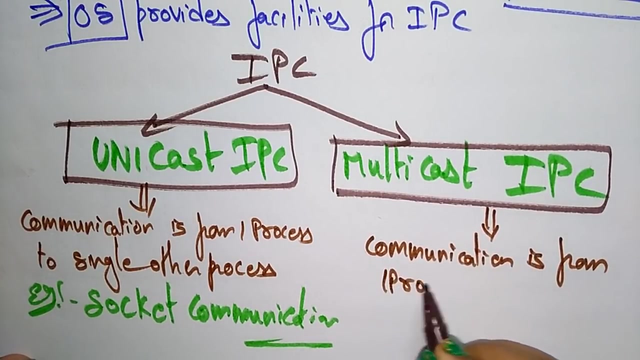 If you connect a socket between two process, then there is a communication exists between those two process That you call it as a unicast. Now coming to the multicast. What do you call this multicast, inter process communication? So communication is from one process to group of process. 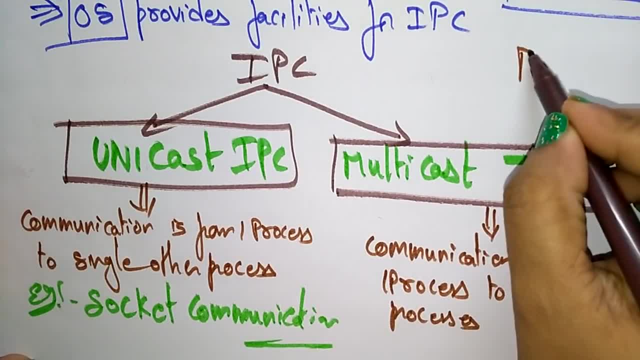 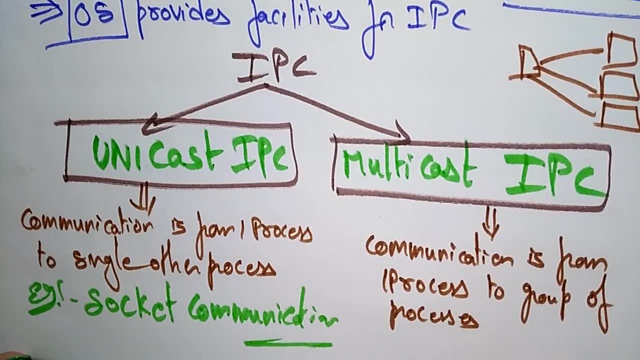 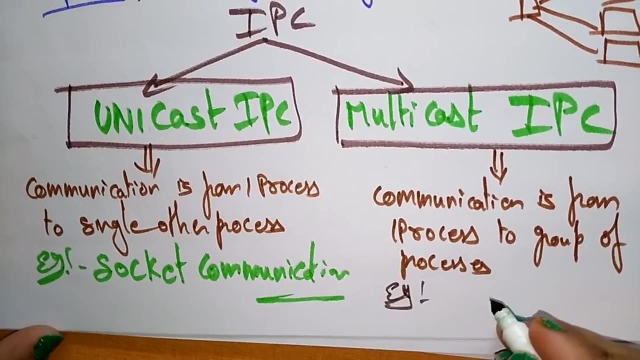 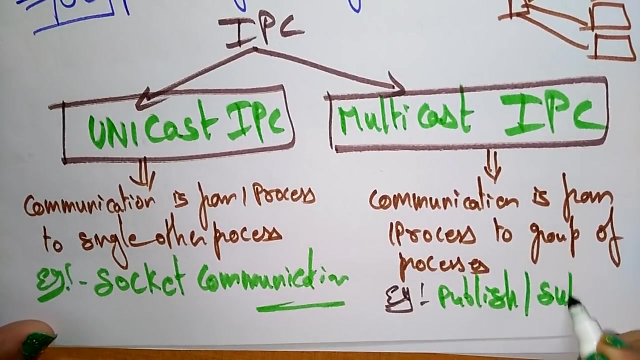 So here I am talking about: one process is going to be communicated with a group of process. This you call it as a multicasting- Multicasting inter process communication. So the example for the multicast inter process communication is: publish or subscribe. Publish or subscribe message models. 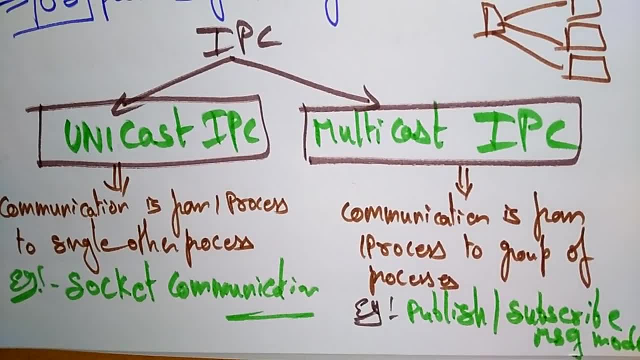 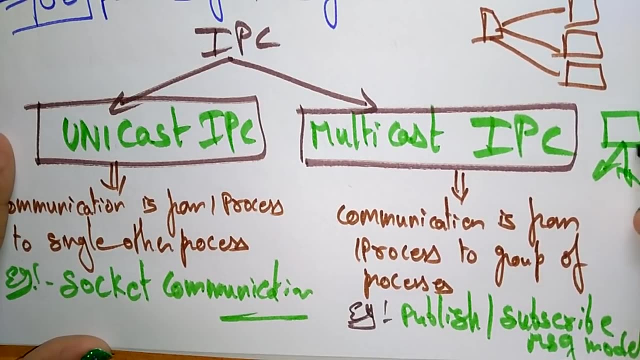 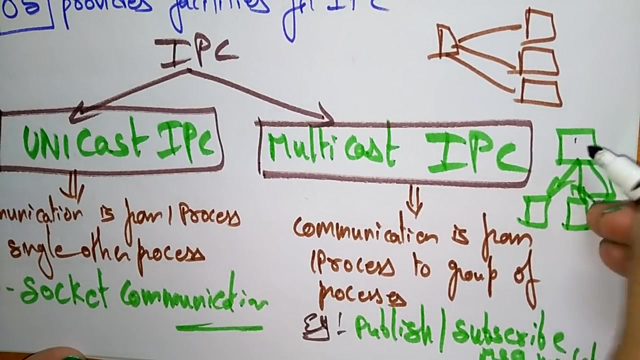 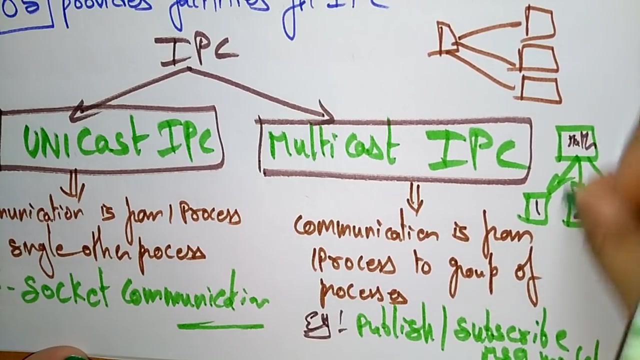 So that you call it as a multicast. Publish or subscribe means: suppose what can I take? Suppose you are broadcast, if you are taking that, So they are publishing. Suppose one Channel is publishing the channel to subscribe, so the different people are going to subscribe this channel. so this is one channel. suppose, whatever the half way, whatever you are taking, so that channel is going to be subscribed by different people, one, two, three different process. so this you call it as a multicasting. so a communication is from one process to a group of process, one process to a group of process. you call it as a multicast inter process communication. 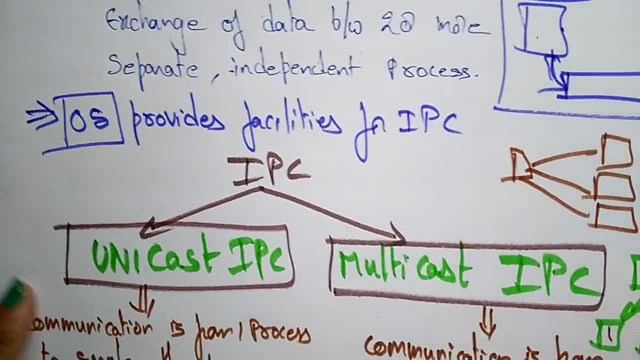 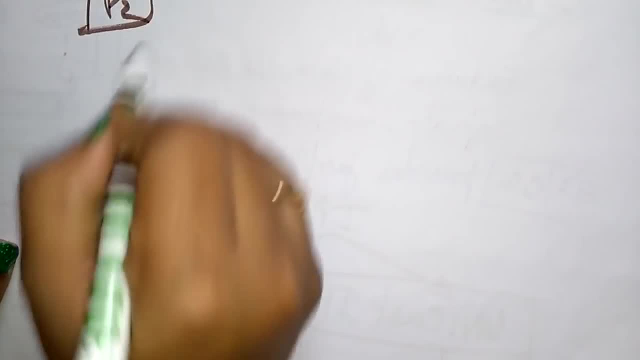 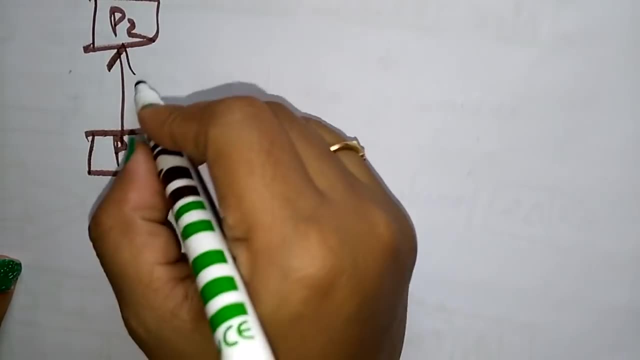 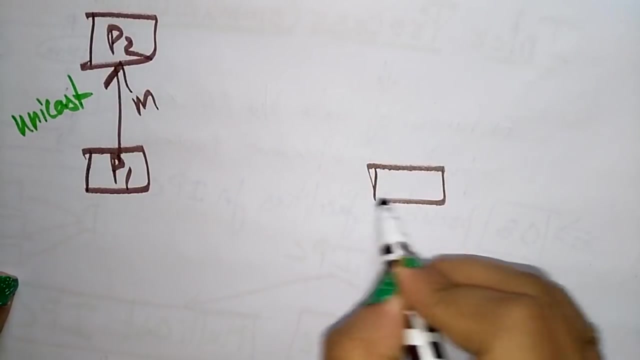 So this, just I am talking about this communication. Suppose this is a process P2 and the P1, if the communication is established between these two process, then you call it as unicast. Okay, suppose if you are taking one process, P1, and these process is going to be communicate with 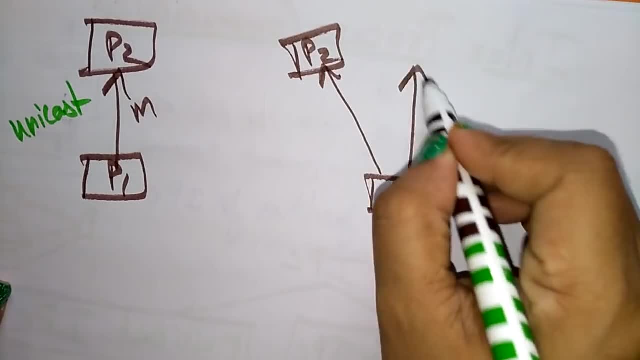 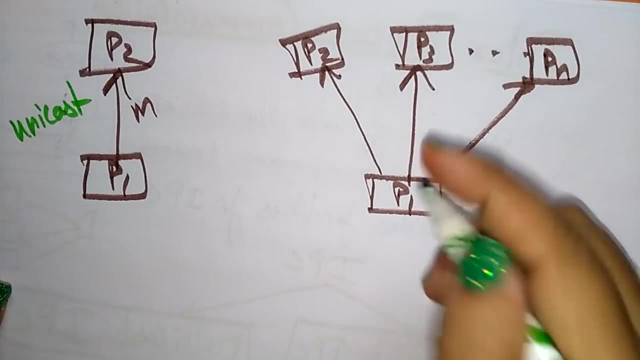 So this is a process P1 and the P1. if the communication is established between these two process, then you call it as unicast. Suppose this is a one type of communication, is Subscription type of communication, then you call it unicast. so then you canся if youare taking all the process. 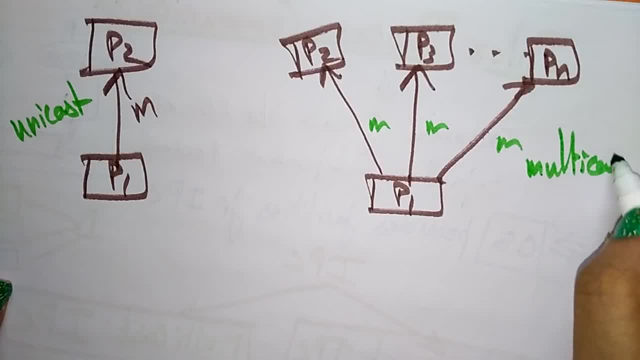 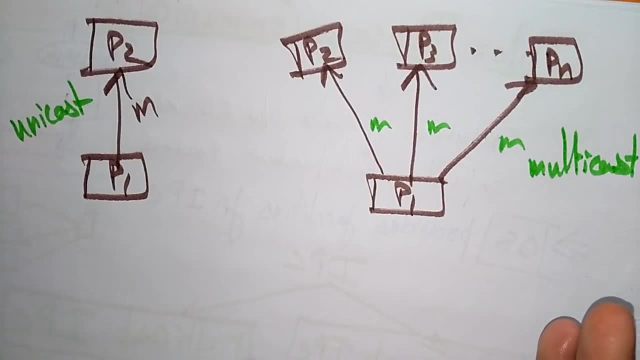 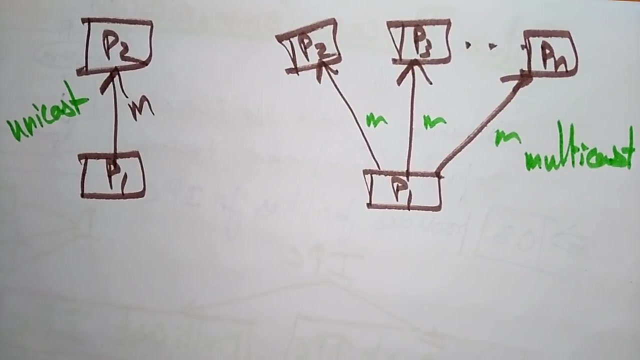 Two or more, Okay so Than these type of interprocess communication. You call it as a multicast. I hope you understand what exactly. Thank you.